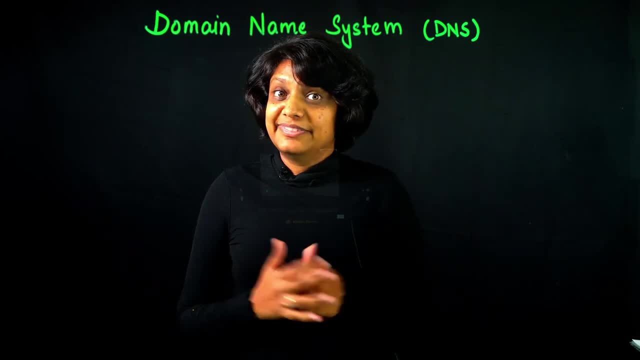 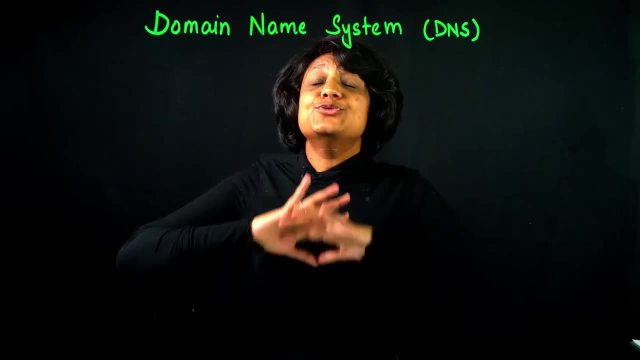 When was the last time you remembered your friend's phone number? Never, right. Well, who remembers phone numbers? That's what contacts in your phone books are for You. save the number in the phone book and then you never have to worry about that number again. 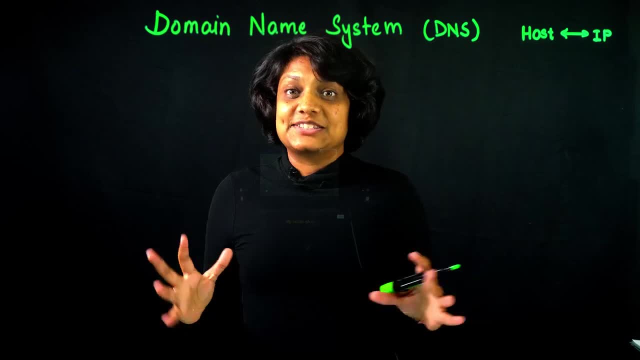 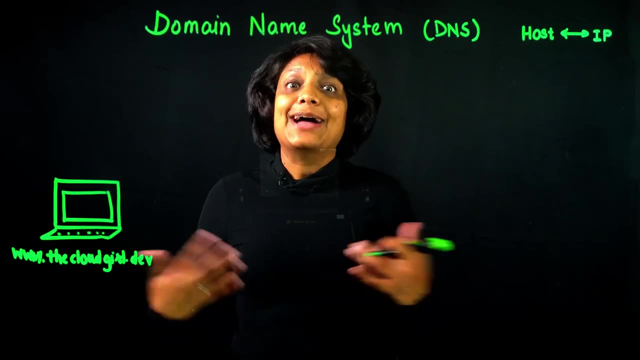 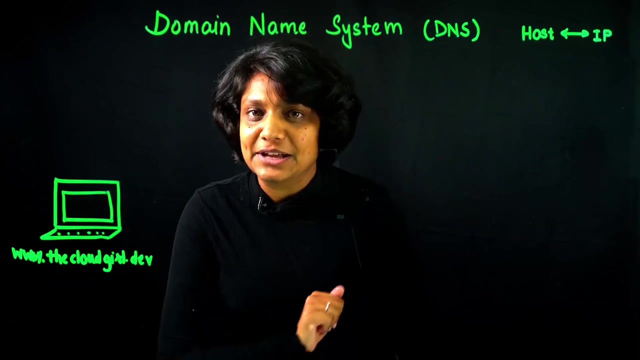 Well, similarly, DNS is a giant contact list of the internet that maps our domain names with the IP addresses. Now, to understand how DNS works, let's consider what happens when we request a website on the internet. Now let's say you type wwwthecloudgirldev in your web browser. 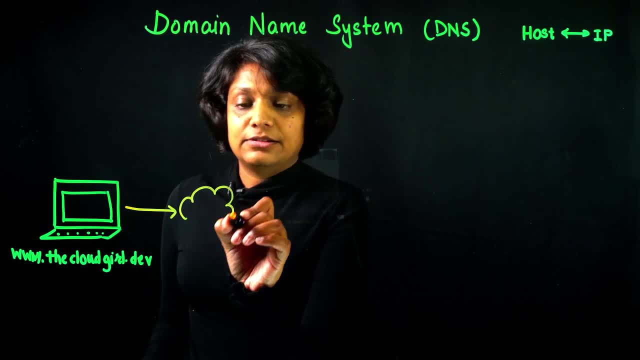 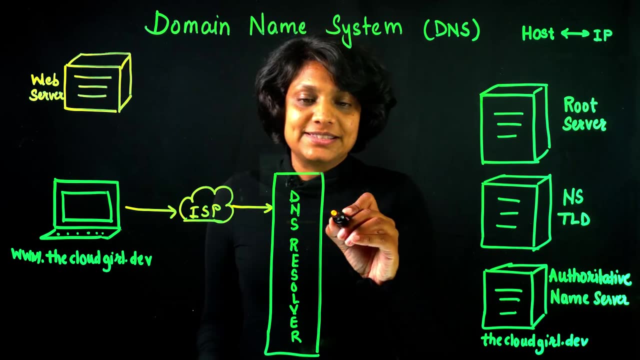 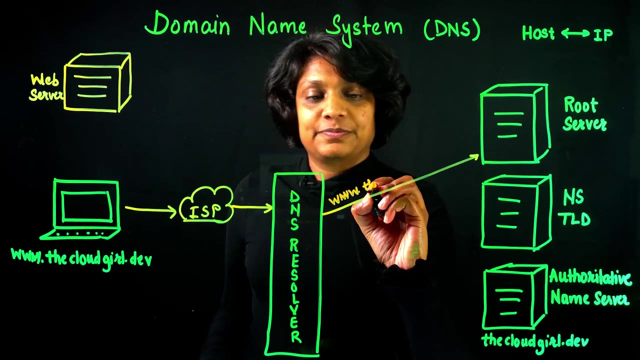 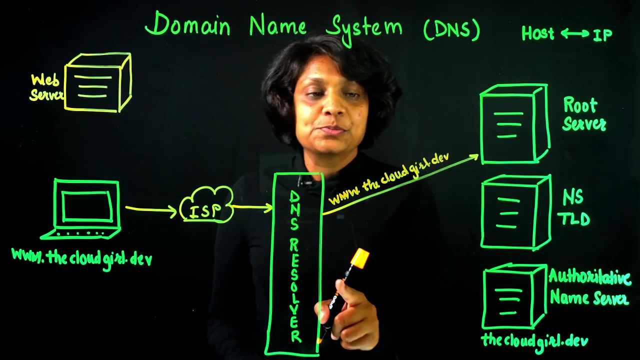 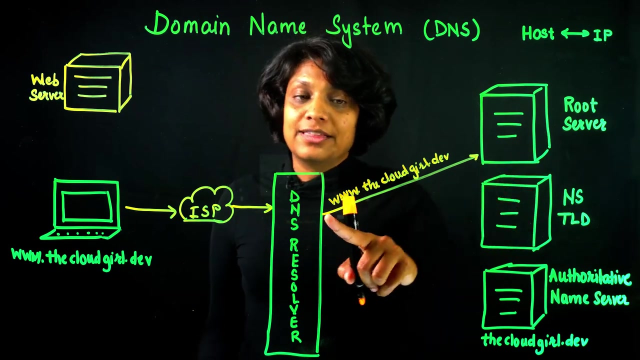 Now your query actually travels the internet and reaches your internet service provider, to the DNS resolver. This resolver then queries the DNS root server with this exact domain, in this case the cloudgirldev, And then the root server basically says that I don't know what the IP address for that is. 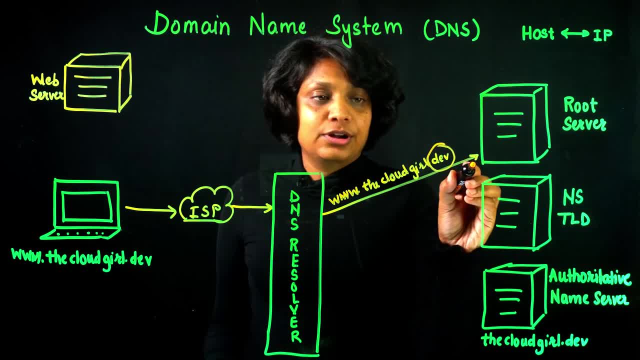 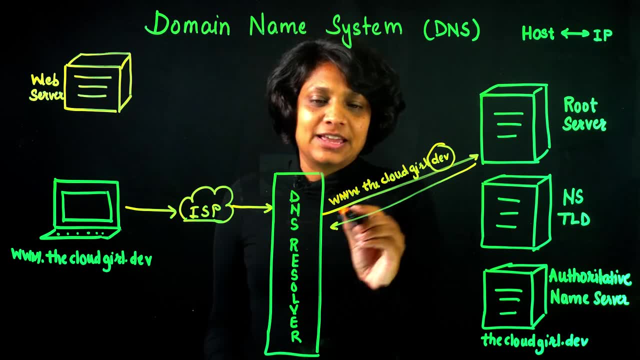 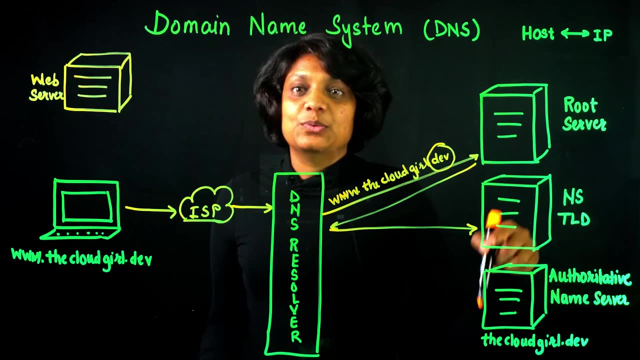 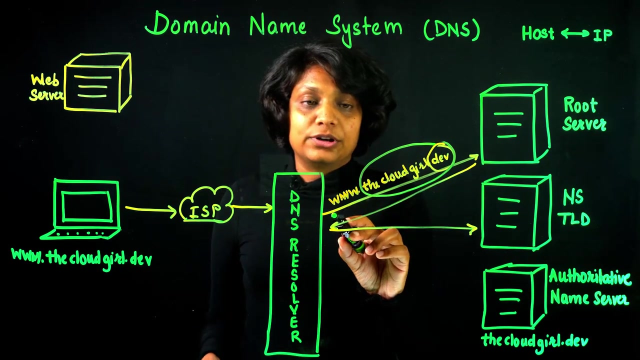 but I do know that you have to go to dev top-level domain name server, which might know what the address is. So then the DNS resolver goes to the dev TLD name server which says it takes this piece right here And it says: I don't really know the IP address for the whole thing. 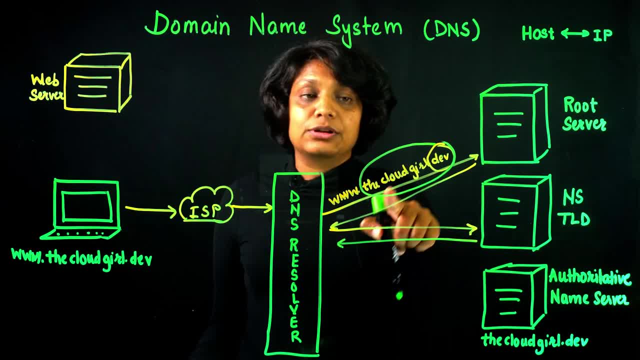 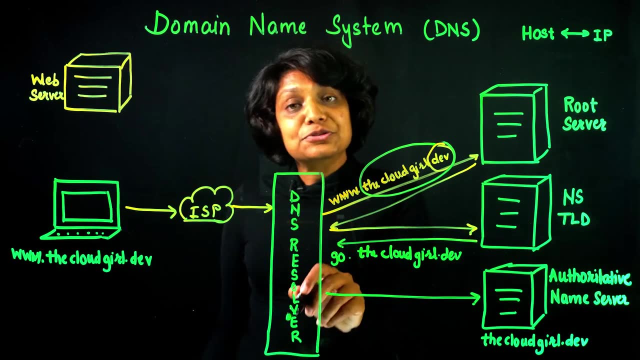 right, But I do know that you can go to the cloudgirldev. you can go to the cloudgirldev domain and that server would know the IP address for www. So then the DNS resolver goes to the authoritative name server for the cloudgirldev. 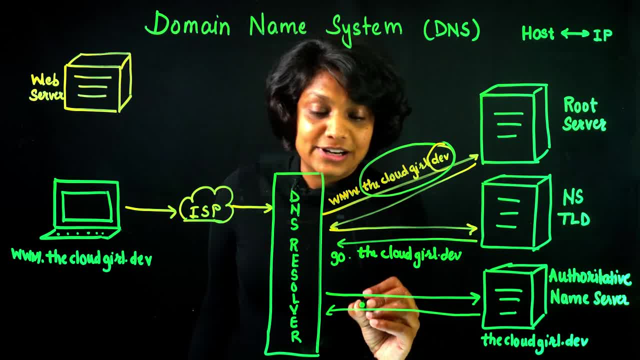 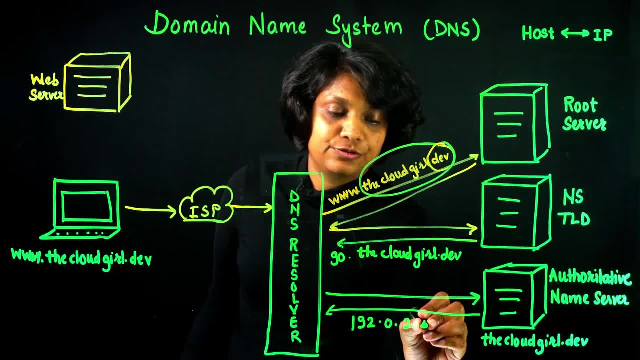 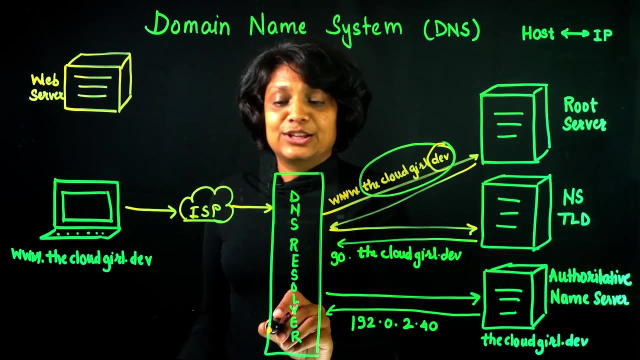 and it returns back the IP address for it, which could be anything, Let's say it's 192.0.2.40, maybe, And then once I have that IP address, the DNS resolver then sends it back through the internet, obviously, to your computer.